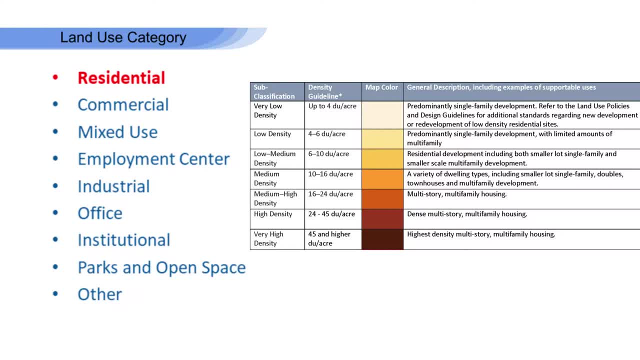 recommendation of 45 dwelling units per acre or greater. It is important to know the recommended density ranges are guidelines and not regulations. There are times when a project may be supported with a higher density than the recommendation. High quality architecture and site design may mitigate the impacts of higher density. 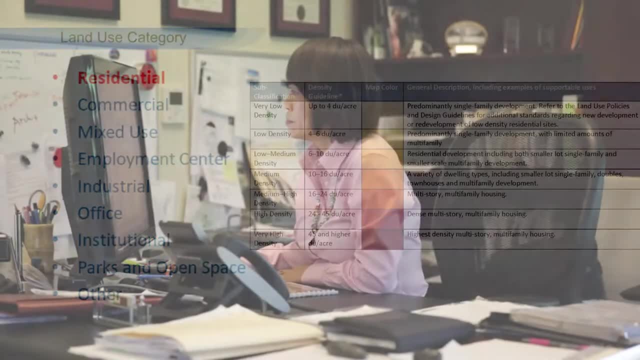 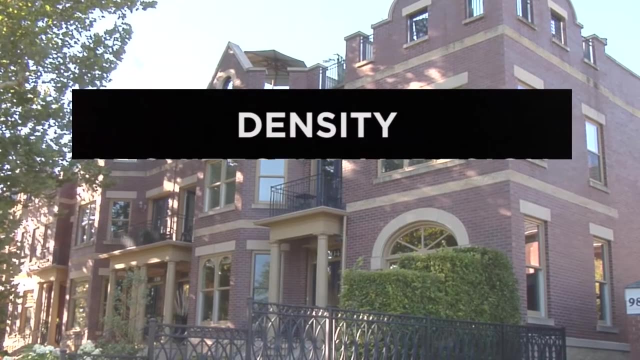 development. in some circumstances, City staff review development proposals for overall consistency with plan recommendations, including density, architectural design and site design. I will quickly review an example of each of the residential classifications for the City of Columbus. The City of Columbus has developed a number of 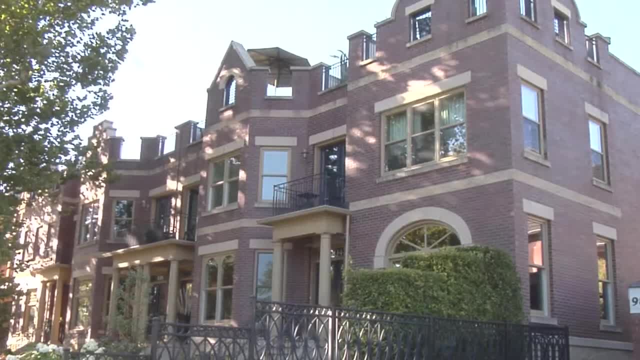 residential classifications, including density, architectural design and site design. I will quickly review an example of each of the residential classifications. However, the 185-s 다음에 a many residential classifications, but remember any type of housing can be found on all residential categories. 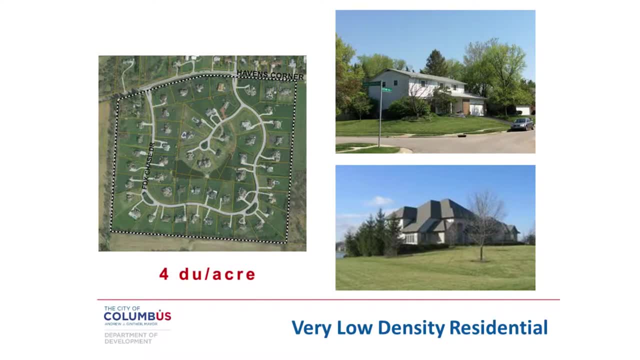 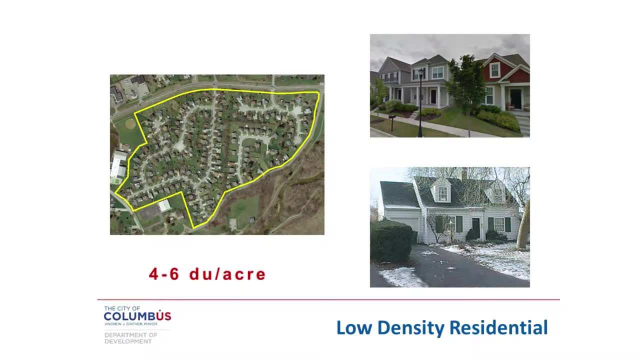 That single unit will hold quite a lot of Welmy Put-in units per year in that example. Very low density recommends up to 4 dwelling units per acre and may be single unit homes. Low density residential recommends 4-6 dwelling units perrons. 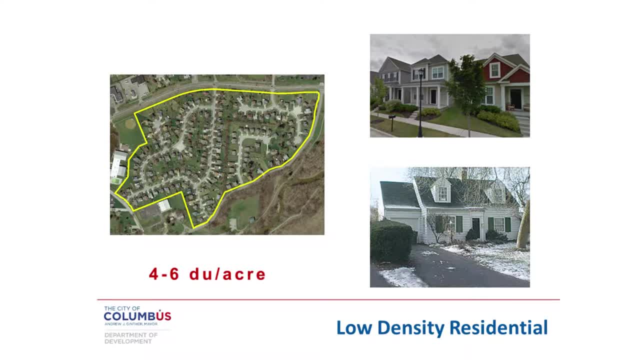 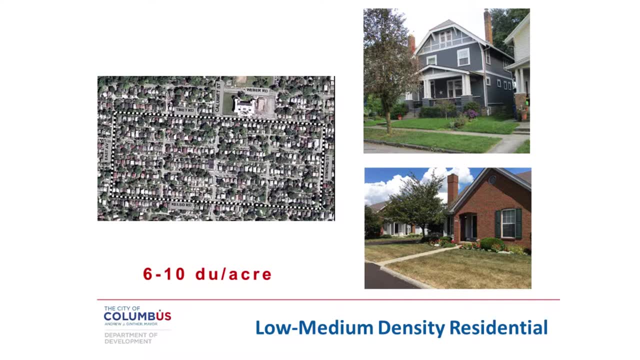 and is typically single unit homes. Low-medium density recommends 6-10 dwelling units per acre and may include smaller-lot single-unit lives. low-medium density recommends 5-10 dwelling units per acre and may include smaller-lot single-unit homes. 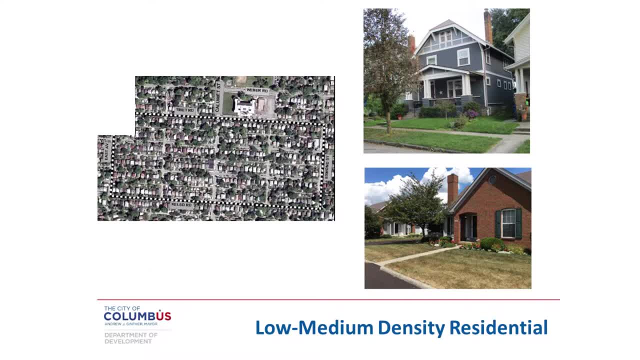 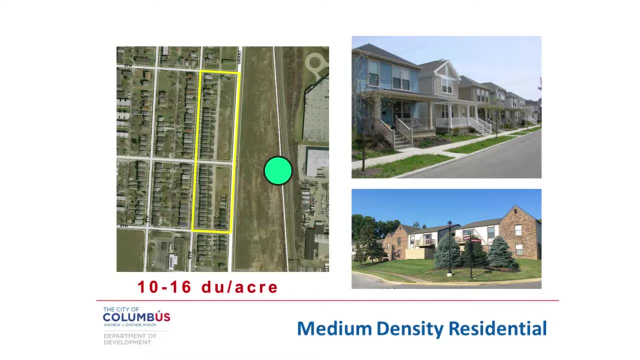 smaller scale multi-unit homes. Medium density recommends 10 to 16 dwelling units per acre and often includes a variety of unit types, including single unit, townhomes and apartments. Again, notice different examples of this classification: similar density, different type of form. Medium density recommends 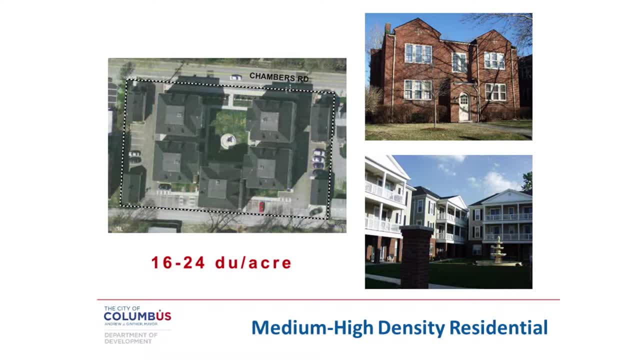 16 to 24 dwelling units per acre and usually includes multi-story, multi-unit housing. It is possible for multi-unit developments to look and feel different with the same density. This is why design is also very important when reviewing development proposals, and we'll discuss this more in the design guidelines video. 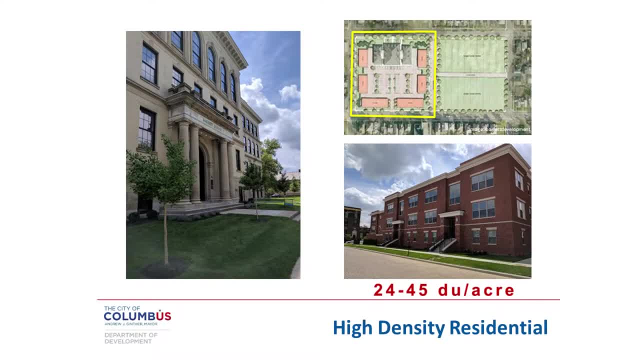 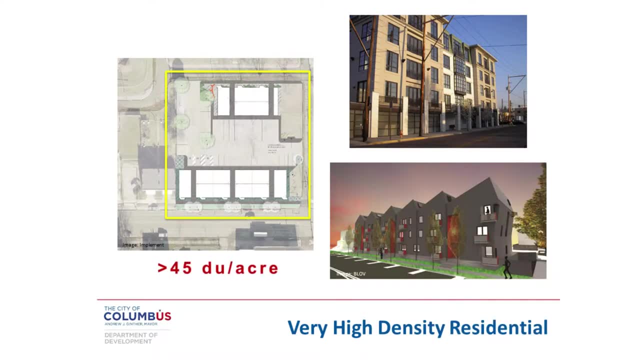 High density residential recommends 24 to 45 dwelling units per acre and is typically multi-story housing. Very high density recommends more than 45 dwelling units per acre and represents the highest density residential case. The mixed use classification allows for a variety of land uses, including 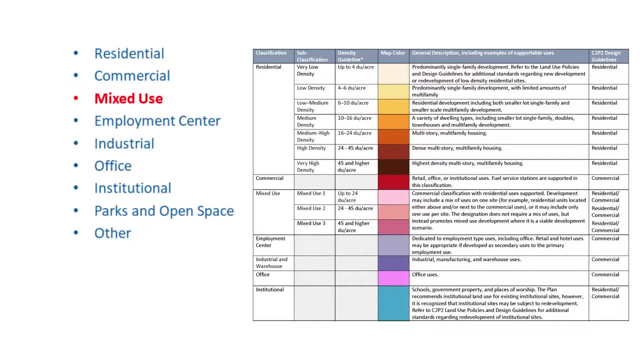 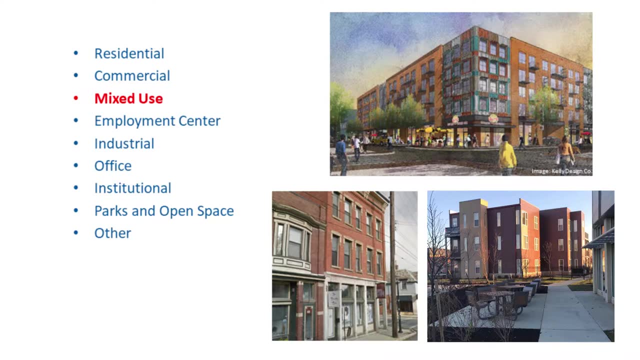 residential, commercial, office and institutional uses. Mixed use policies encourage a mix of uses within an area but do not require a mix of uses. Generally, mixed use is recommended along primary corridors and within established commercial centers. Similar to the residential categories, there are three. 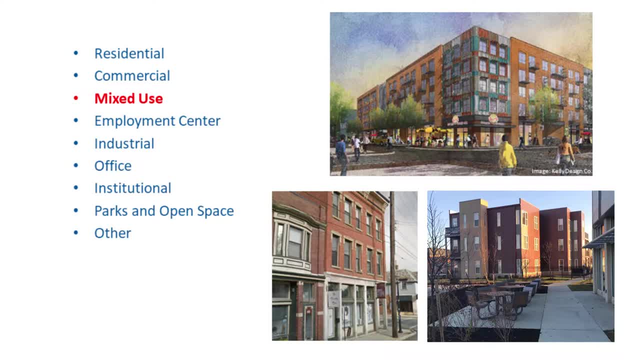 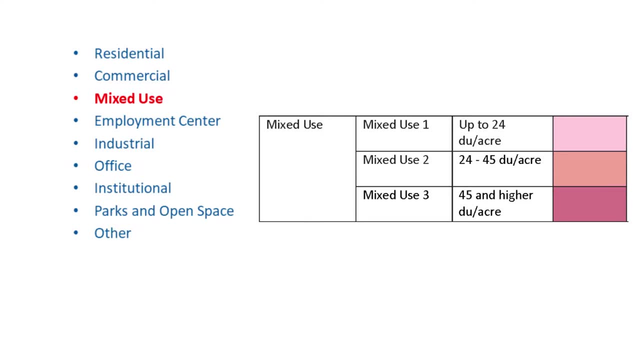 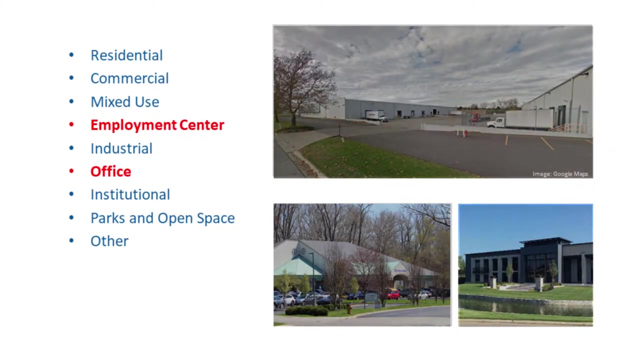 mixed use. categories that are classified as mixed use. We recommend mixed use classes only for residential, commercial or residential use. Vaud, where supportras are not classified by density. to account for residential development mixed-use one recommends up to 24 dwelling units per acre. mixtuse two. 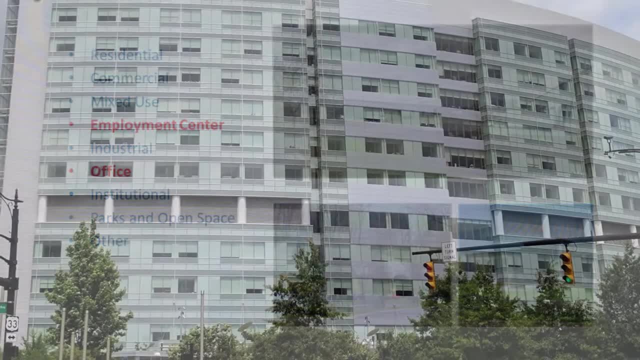 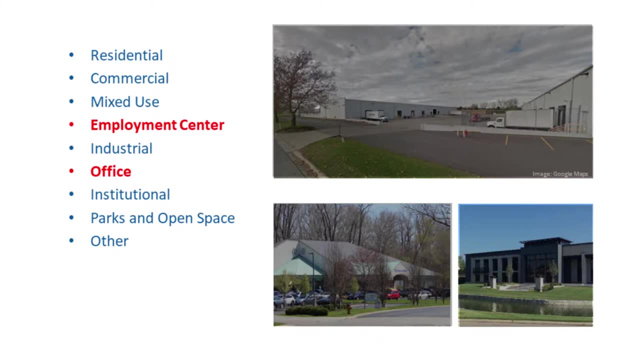 recommends between 24 and 45 dwelling units per acre and mixed use. 3. recommends greater than 45 dwelling units per acre, appropriate in certain cases and generally. retail and residential uses are not supported in this category, but retail may be appropriate as a secondary use to the primary business. 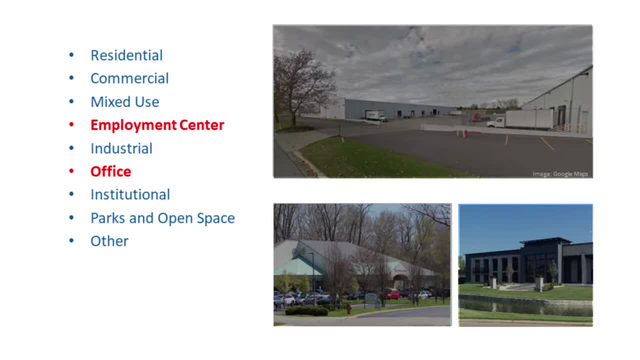 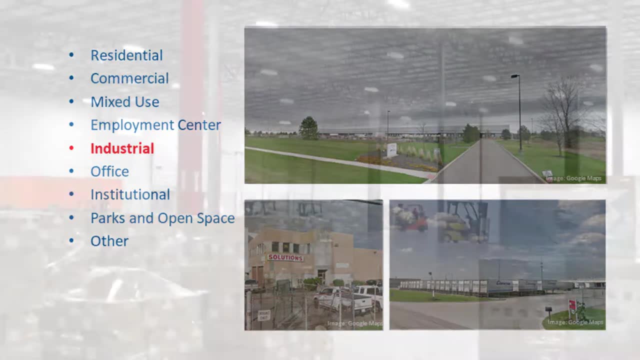 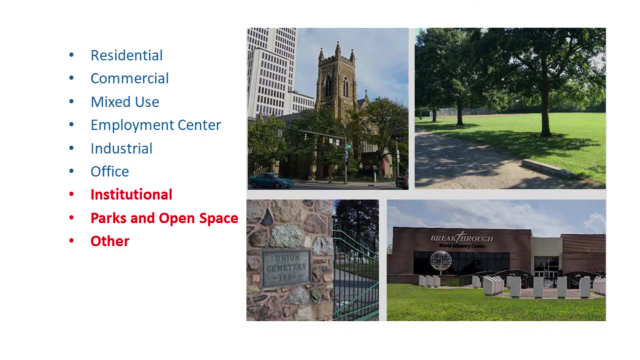 the office classification applies only to office uses. the industrial and warehouse classification includes industrial, manufacturing and warehouse uses. several of the land use categories are only applied to existing land uses. these include institutional parks and open space classifications and all land use categories listed as other on the classification table. 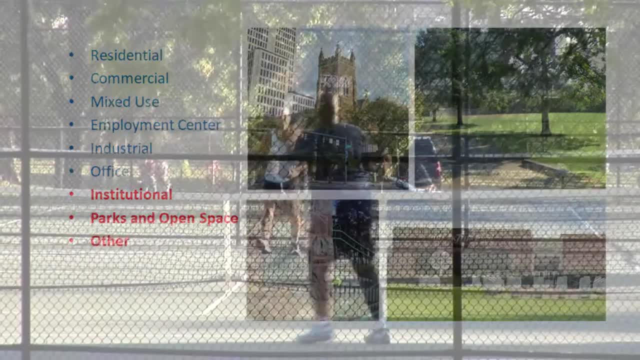 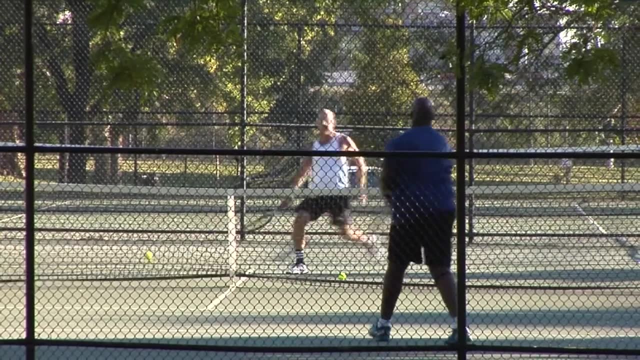 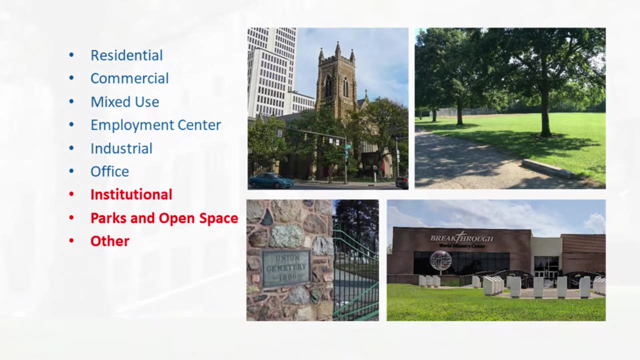 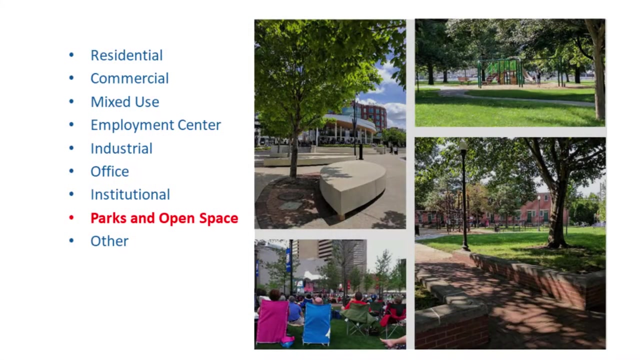 while our land use plans do not provide site-specific recommendations for new institutional uses or parks and recreation, these uses are addressed through the policy text and are generally supported in most areas. the institutional classification applies to schools, government property and houses of worship. there are three parks and open space classifications, including parks and recreation, open space and private open. 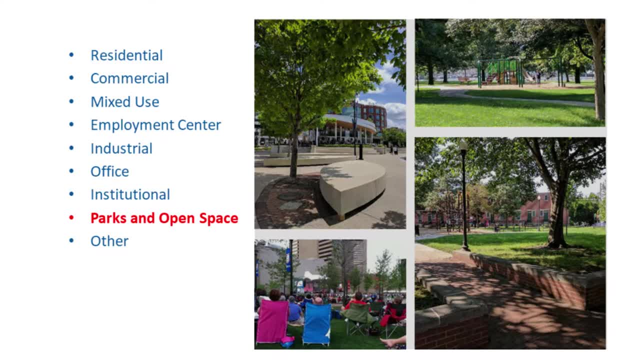 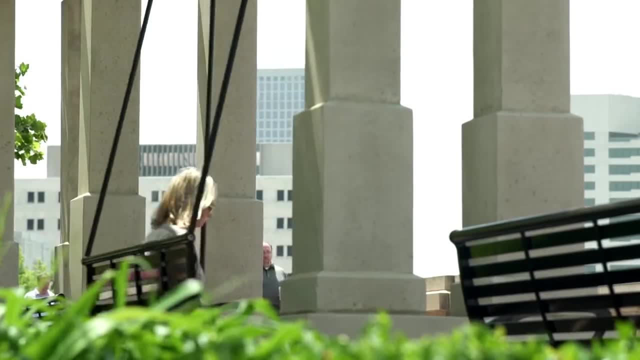 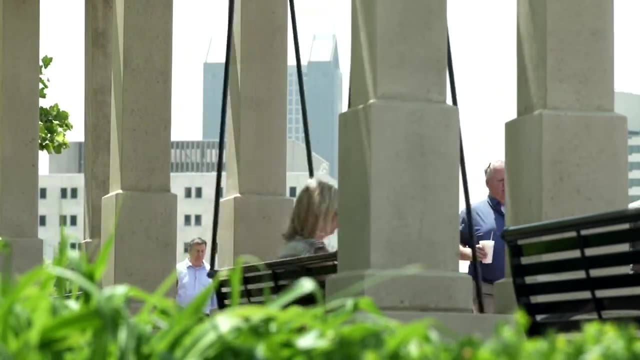 space. the definitions for each classification are provided on the classification table, which is available online. once again, instead of providing site-specific recommendations for parks within a land use plan, the c2p2 land use policies and design guidelines recommend consideration of parks and open space in appropriate areas. 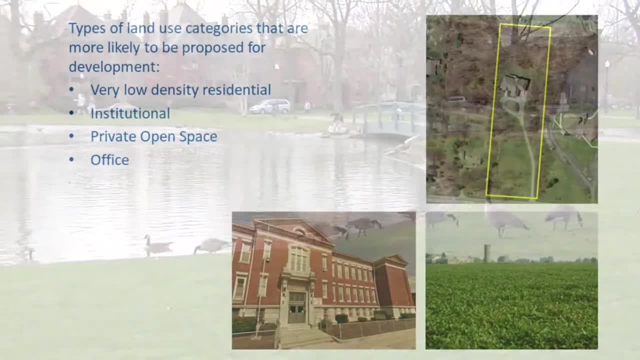 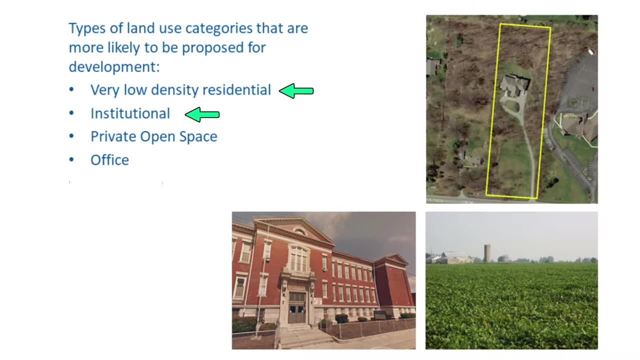 some existing land uses are more likely to be proposed for development than others, including very low density, residential, institutional, private open space and some existing office uses. generally speaking, these types of existing uses are recommended to remain the same in the plan, but there may be other uses that are appropriate for the sites too. 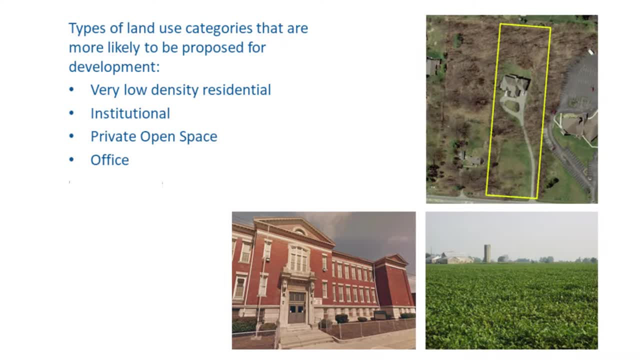 in order to address this issue, the land use policy text for these categories includes guidance on how to review development proposals that are not consistent with the plan recommendations. we will talk about this more and review some examples of this in the next section, when we talk about land use recommendations. 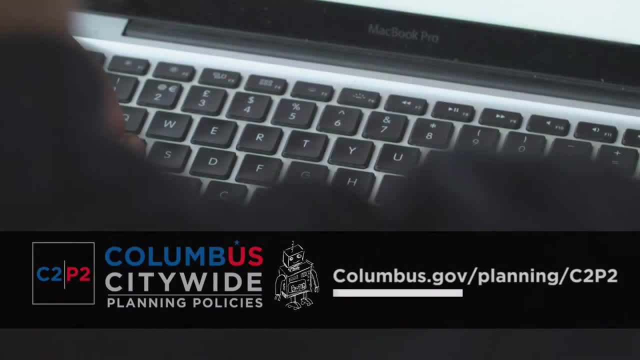 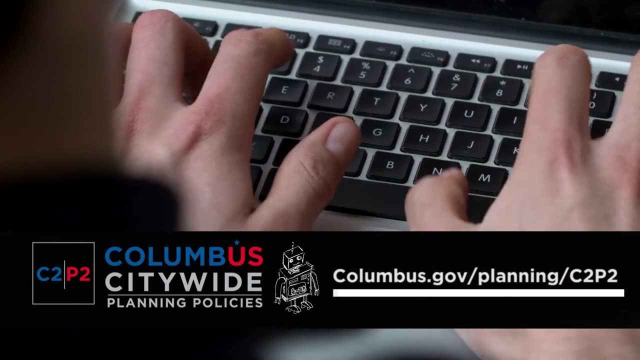 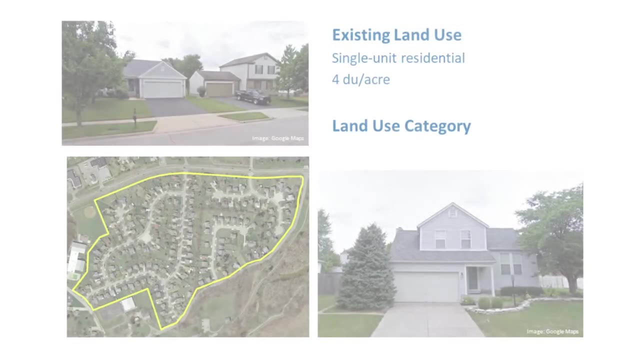 we are now going to show a few existing residential developments and ask you to determine the correct land use category. if you'd like, you can download the land use classification table and use it to assist you with the exercise site. example number one is a single unit residential. 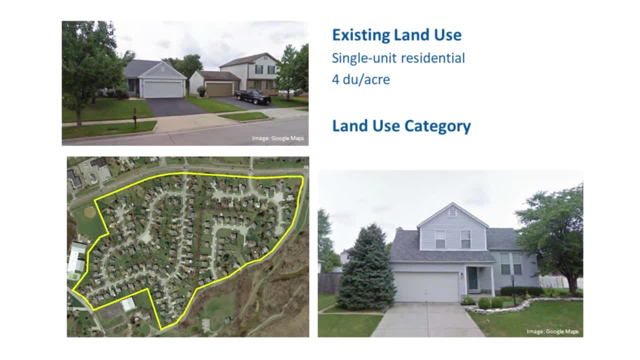 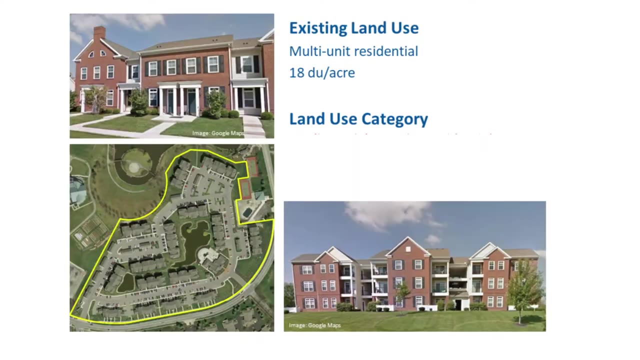 development at a density of four dwelling units an acre. what is the correct land use category? the correct answer is low density residential site. example number two is a multi-unit residential development at a density of 18 dwelling units an acre. what is the correct land use category? 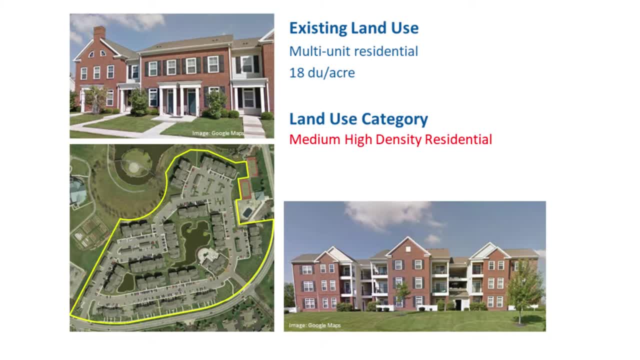 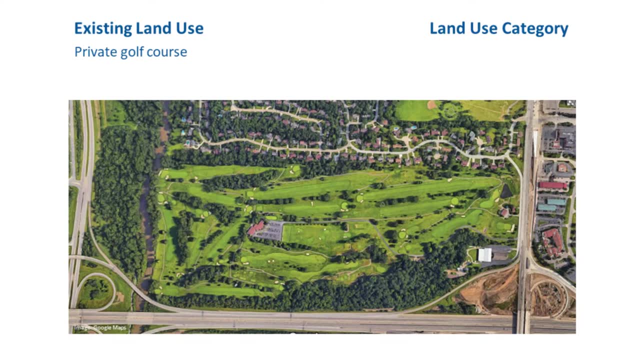 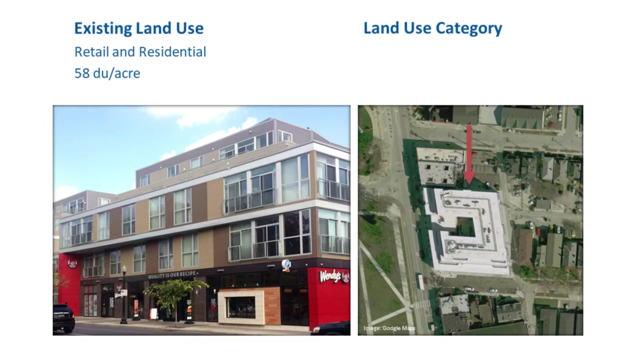 the correct answer is medium high density residential site. example number three is a private golf course. what is the correct land use category? the correct answer is private open space site. example number four includes both a retail and residential use. The residential use is 58 dwelling units an acre. What is the correct? 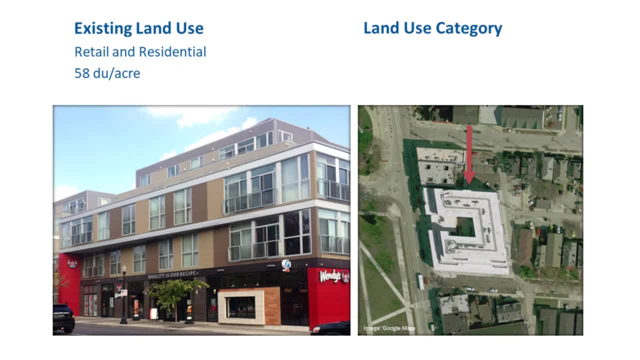 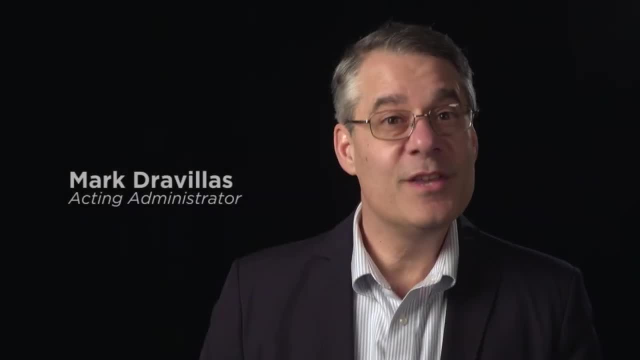 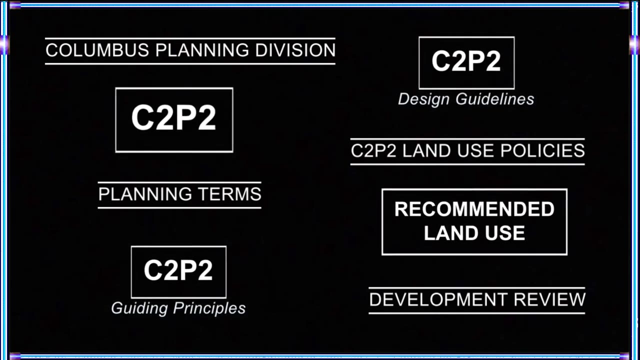 land use category. You are correct if you answered mixed use three Congratulations. Thank you for completing this video on land use policies. Please continue to the next video to learn more about how land use recommendations are determined.